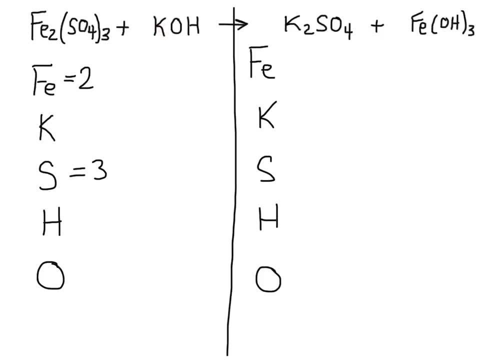 And then we have just one potassium. So there's the K as potassium, We have one hydrogen, One by itself there, And then the last thing to count here is the oxygen. So there's four oxygen inside these brackets. We're multiplying that by three. 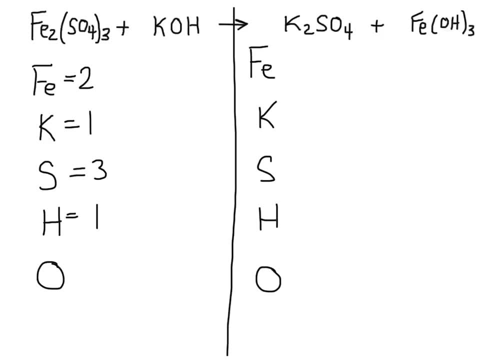 So there's really Twelve oxygen here. plus that one is 13 oxygens. Now let's count up the other side. So we have just the one iron here. We have two potassium. So here's our K, with the two next to it. 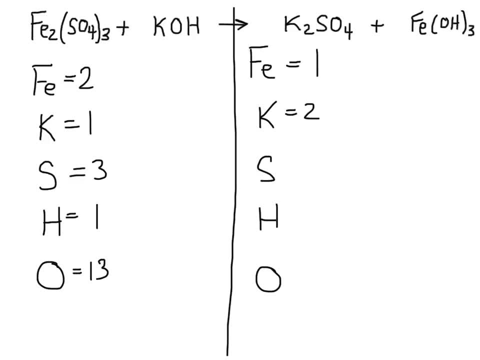 So it's two potassiums. We just have one sulfur. There's sulfur, just one of them. We have three hydrogens, So here's the one hydrogen inside the brackets And we're multiplying that by three, So there's three hydrogens. 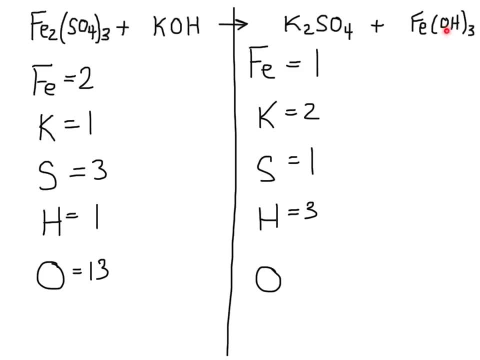 And then, finally, we have three oxygens over here, So one oxygen times three, plus these four oxygens over here, So that's seven oxygens. Now the goal of balancing is that we get these numbers to equal for each of these elements, So both of those should be the same. 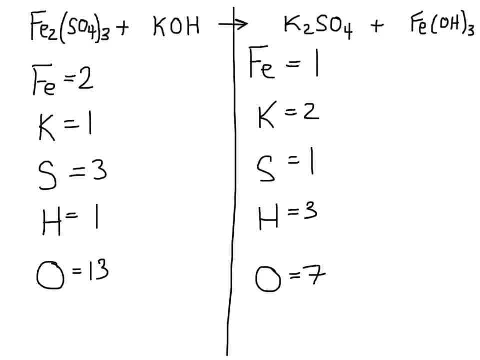 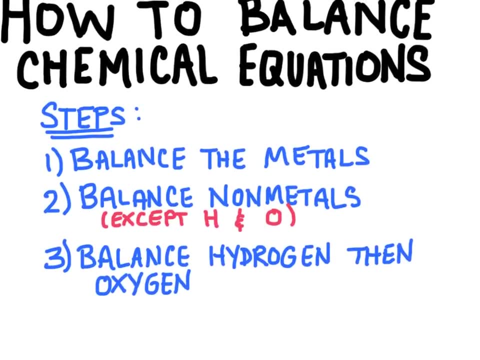 Both of those should be the same, and so on. So that's our goal. Here are the steps to be able to reach that goal. These are steps to balancing chemical equations. The first, The first step, is that we're first going to balance the metals. 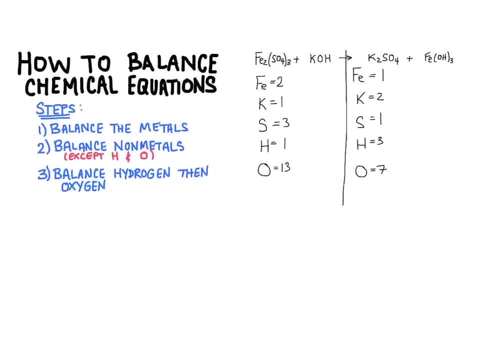 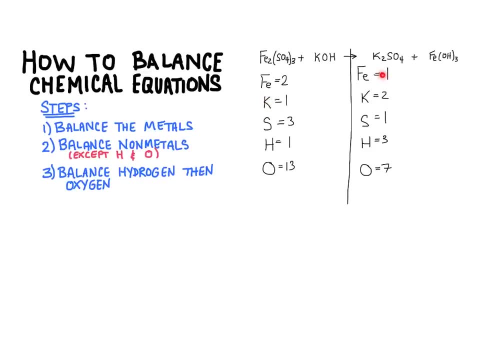 We're going to make sure the metals balance each other. So, as I'm looking at this equation, I have two metals, I have iron and potassium. I'm going to start by getting those numbers to equal, Then I'm going to move on to the non-metals, except for hydrogen and oxygen. 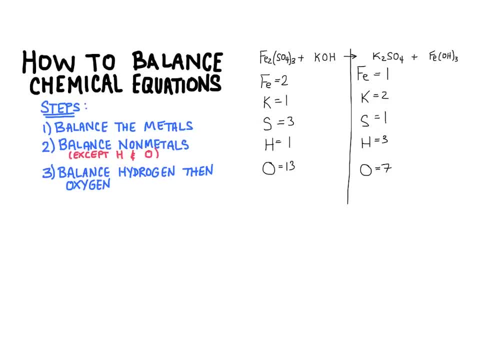 The only thing I have other than hydrogen and oxygen- that's a non-metal- is sulfur. Finally, I'll balance hydrogen, then oxygen. So you see, I listed them in the order that I'm going to follow these steps. So how do we go about changing these numbers? 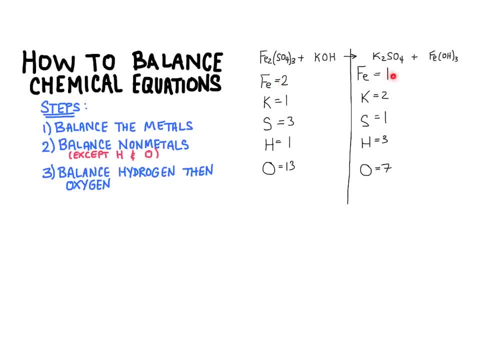 I have two irons here. I have one iron here and I want that to be two. I want these to match. The one thing I cannot do is I can't change these subscripts. So that little two. I can't just simply put a little two in there. 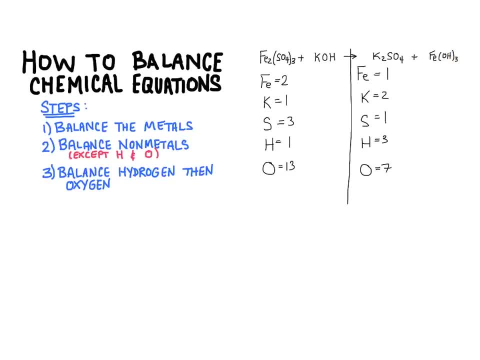 These things, right here, are set in stone. What I can do is I can change the coefficients, and that's numbers in front of these chemical compounds. So right here, there's nothing there. but since there's nothing there, we just assume a one is there. 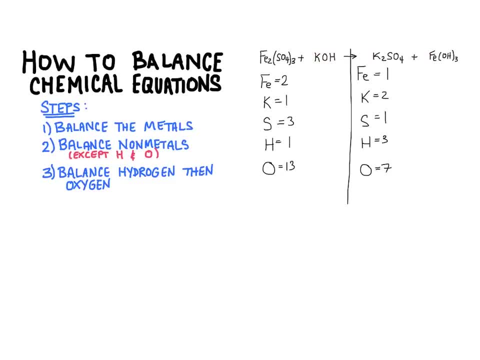 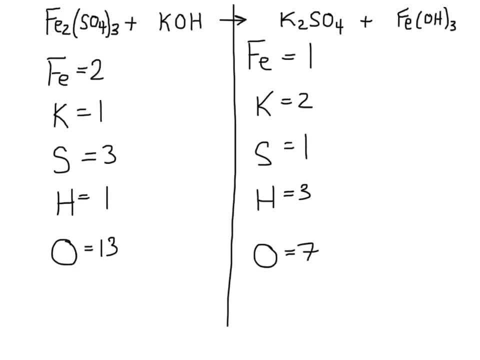 We've got to change these amounts of each of these molecules, or these compounds, I should say, because we want these numbers to all balance each other. So here's the first thing I'm going to do: I'm going to put a two right in front of that iron hydroxide. 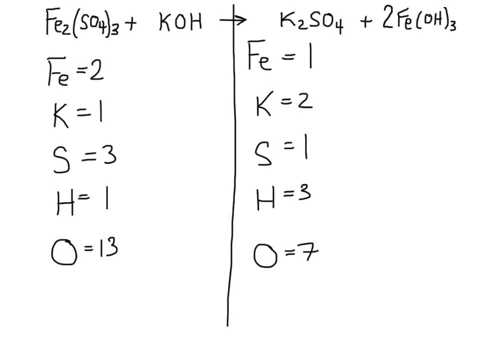 So I'm going to put that two there. That's going to change not only the amount of iron, It's going to multiply everything here by two. It's really like I have two of these compounds, the whole thing. So it's going to say that I have two irons, but it's also going to change the amount of oxygen and hydrogen. 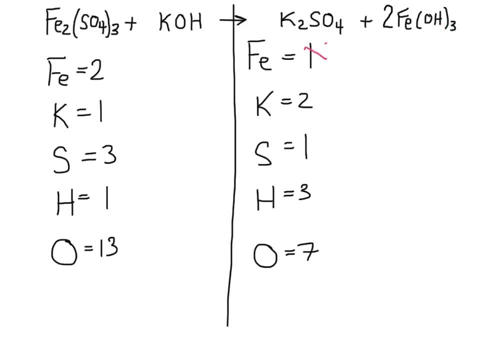 The first thing I'm going to do is I'm going to change this one to a two, because now I have two of them And then I need to go about and check: well, what else did I change when I put that two there? 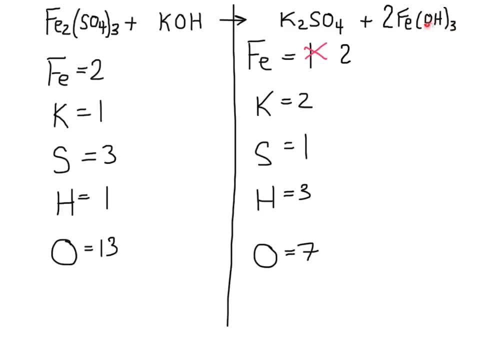 Right here the oxygen. I had three of them right, because it's three times everything inside the brackets, And then I'm multiplying that by two, So I really have six oxygens here. I can't forget about these ones over here. 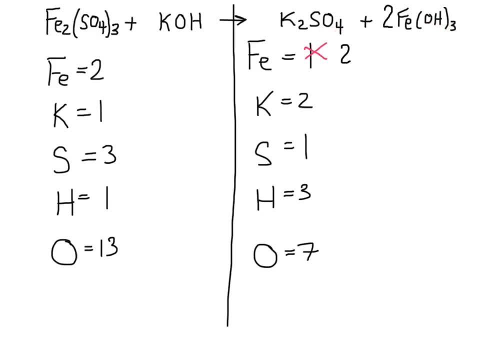 So that's six plus four. So I have changed the number of oxygen from seven to ten. That's the six plus the four. I also changed the number of hydrogens. So over here was hydrogen. There were three of them. I'm multiplying that by two. 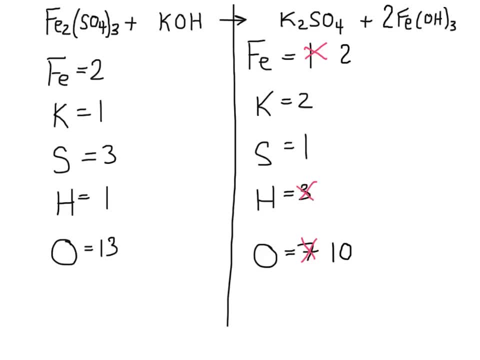 And so I'm going to change this three now to a six. Now, I should have mentioned this earlier. Make sure you use a pencil when you're putting in these subscripts, because this could change. We're going to keep on adding coefficients here. 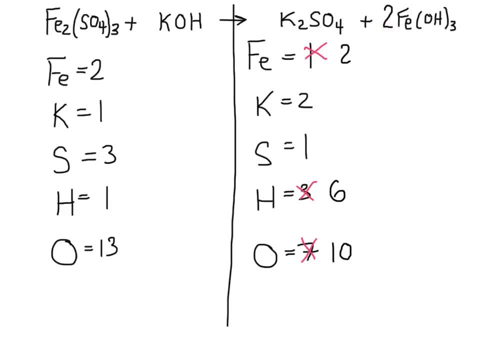 So we might have to change this later. So use a pencil, because we might have to change that. We'll see what happens. Now that the irons are balanced here, remember, step one is I want to balance the metals. The other metal is potassium. 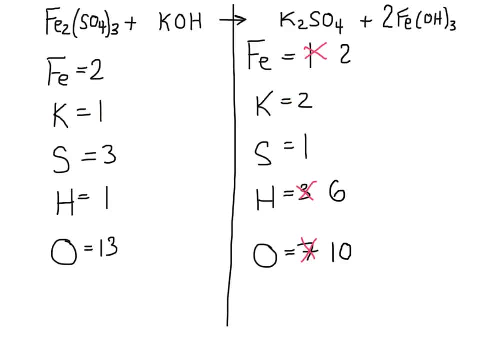 I need to balance this as well, So I'm going to look on this side. I have one. Here's KOH. I'm going to put a two in front of that. So we're going to change this number from one Now two. 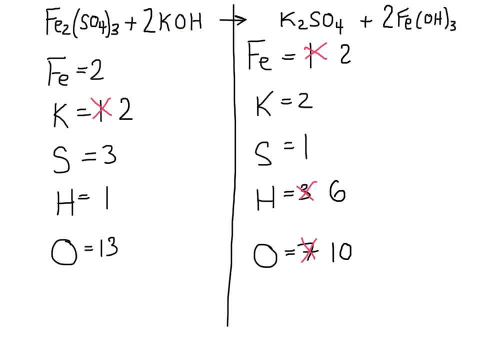 And while I did that, I changed the amount of oxygen and hydrogen, So I need to account for that as well. First, we'll start with the hydrogen. There was one. I'm multiplying that by two, So now I have two hydrogens here. 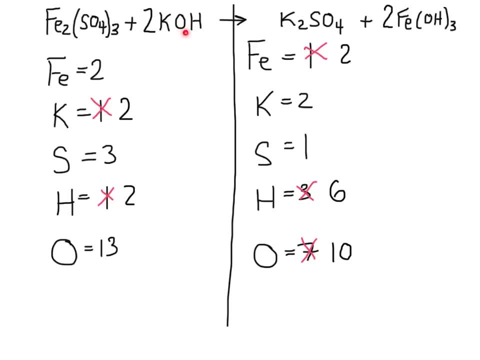 And I also changed the amount of oxygen. There used to just be one oxygen here. I multiplied that by two, So there's two oxygens here in this area. Over here I had 12.. So that's a total of 14 oxygens now. 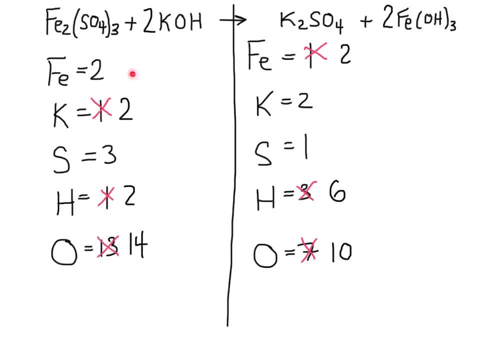 I'll change that as well. Now I can double check my metals. Metals are balanced. Now I can move on to the nonmetals, except for hydrogen and oxygen. I'm going to leave those till the end. So now we're at the sulfur. 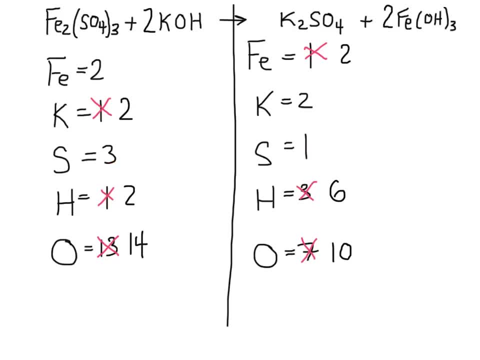 Three sulfurs on this side. I only have one here, So I am going to add a three where I see sulfur. So here's the only spot I see the sulfur, So I'm going to put a three right here. Now it's going to triple all of this stuff in here. 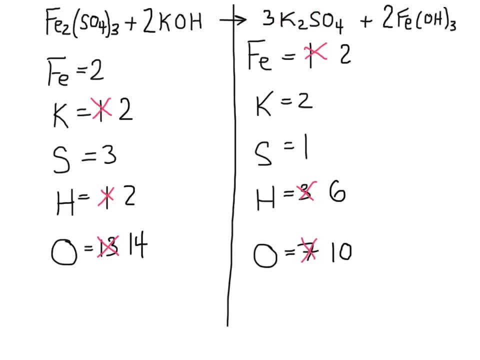 So there's only one sulfur in the compound, but I'm multiplying that by three, So I'm going to add a three. So I'm going to change this from one to three, But I've also changed a lot of other things here. 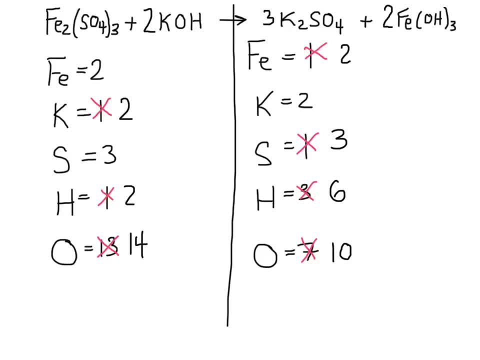 So I want to check what I did. There were just two potassiums here, but I've multiplied that by three. Now I'm at six potassiums on this side. Looks like we're throwing things off from what we just did. It looks counterproductive, but it's not. 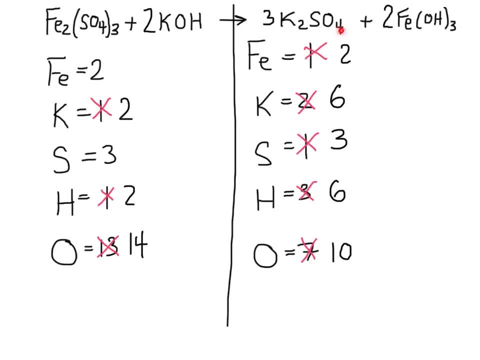 Hang on, We're going to get there, And I've changed the oxygen as well. There used to be four oxygens right here. Multiply that by three, so that's 12.. And then over here I have six, So we're at 18 oxygens on this side now. 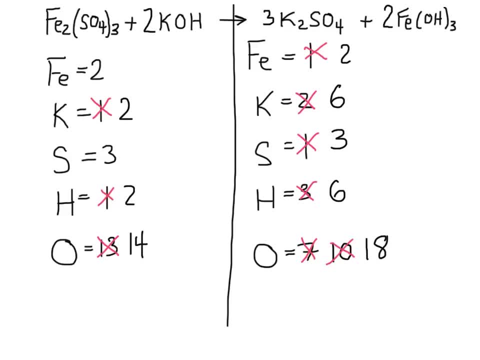 So I'm going to change this number And I'm going to check here to see. my sulfurs are balanced, My irons are still balanced, but now my potassium is not, So I'm going to go back. I don't want to move on to the step.